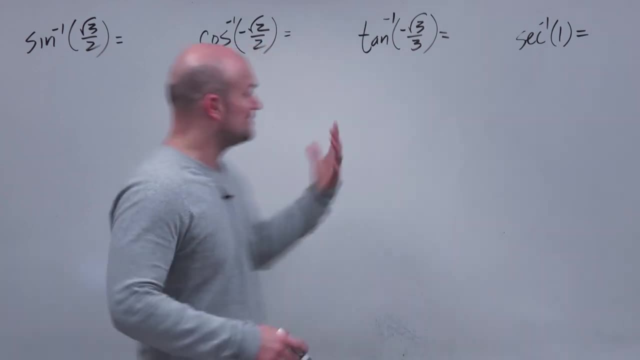 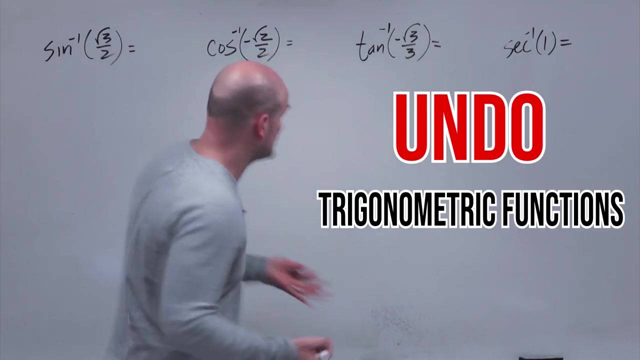 inverse trigonometric functions, as well as the restrictions and why they are going to be used. So the first idea is: you know these inverse trigonometric functions, we use them to undo the trigonometric functions. So to understand what we're looking for, it's best to kind of 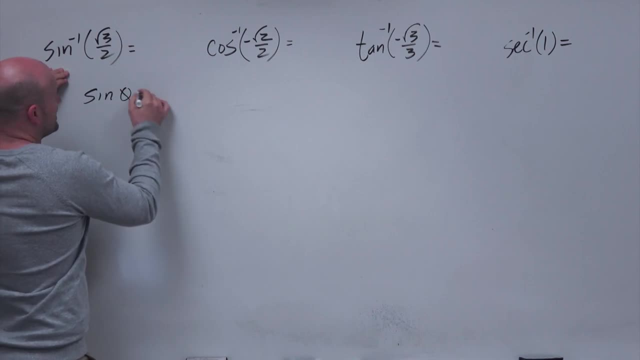 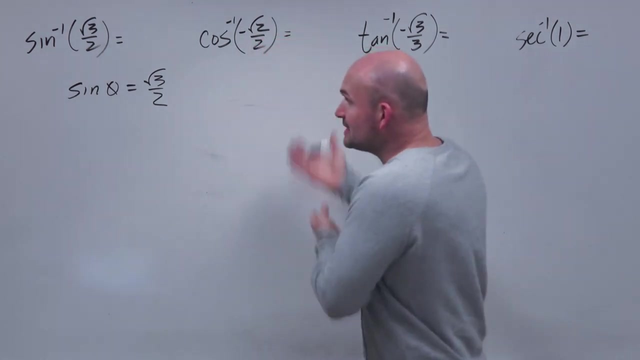 look at this as an equation. If I said the sine of theta is equal to the square root of three over two, right, what I'm saying is the sine of what angle is equal to square root of three over two? Now you could think of the square root of three over two as opposite over hypotenuse, but once. 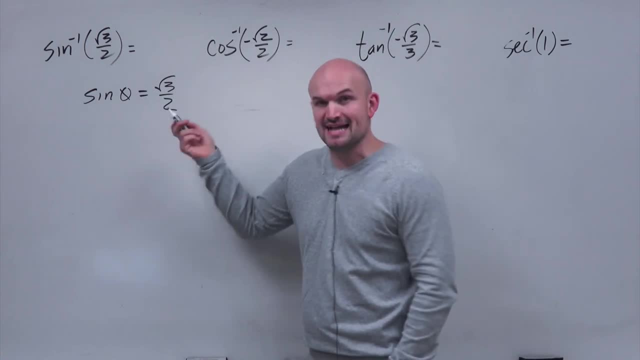 we've evaluated from the unit circle, we like to think of the sine as the y-coordinate of that point on the unit circle, because obviously those coordinate points are created from triangles. So if I'm thinking about this, I say, all right, well, when is the sine of theta equal to square? 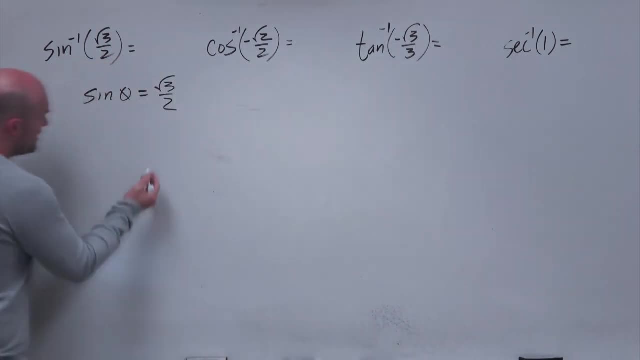 root of three over two right. So just thinking about this and we say, well, if we go ahead and take a look at the unit circle here, we recognize now that there's actually a point right here And we can say: all right, that point, that. 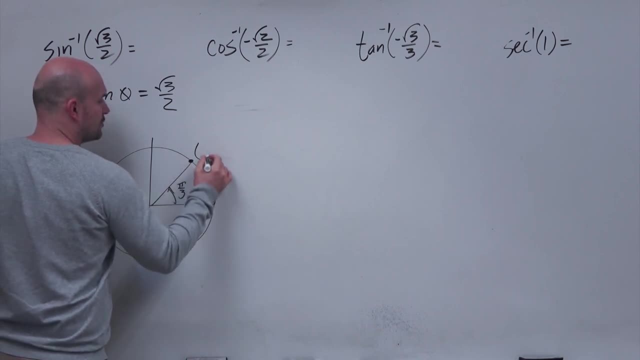 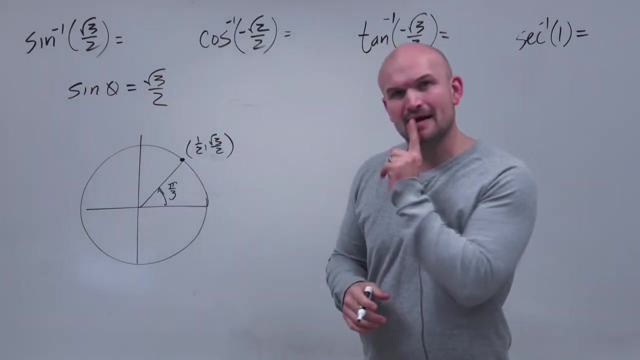 one's pretty easy. that is going to be pi over three, because this coordinate point is going to be one half comma, square root of three over two, right Done. But then we start to think we say, oh, wait a minute, I think there's more points. What about this? 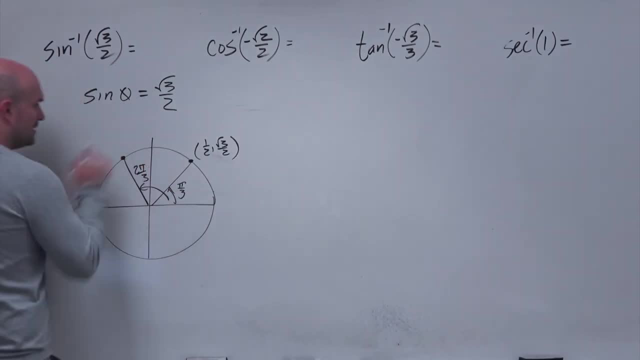 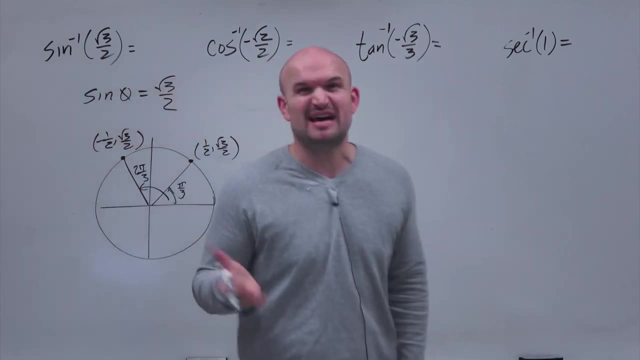 point over here, What about two pi over three? Because that point just has a negative x value but it still has a positive y value, And say, okay, well, we have two values, like we can have two answers, right. And then we say, well, wait a minute, what about negative five pi? 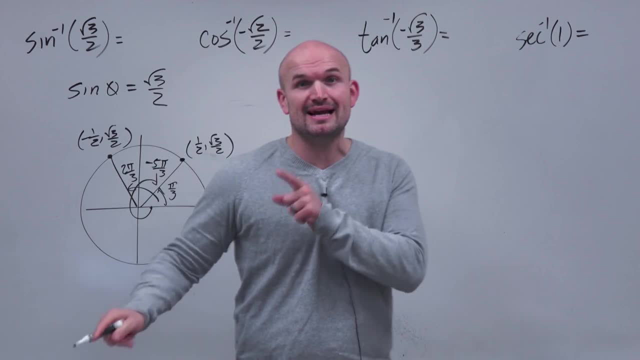 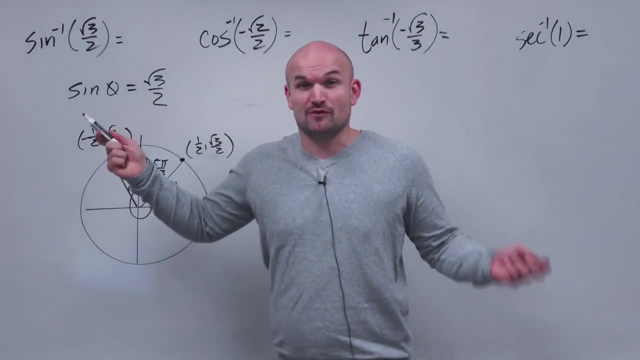 over three. Well, that works. And then we start going down coterminal angles and we recognize that we can keep on going around, and around and around the circle. So if we're not looking for one angle, we're actually looking for infinite many answers. So the 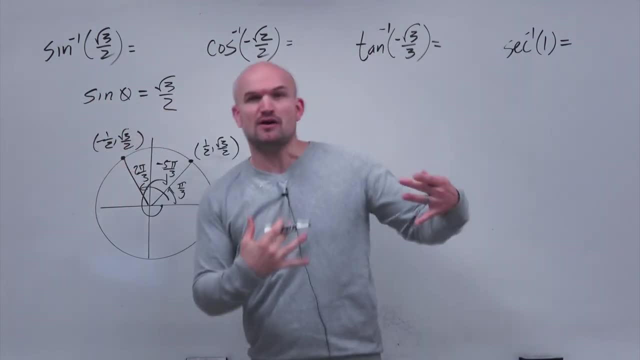 problem doesn't come back with this equation, because that makes sense for an equation We can solve. for an equation with multiple solutions. The problem comes into when we're dealing, when we're trying to evaluate the equation we can solve for an equation with 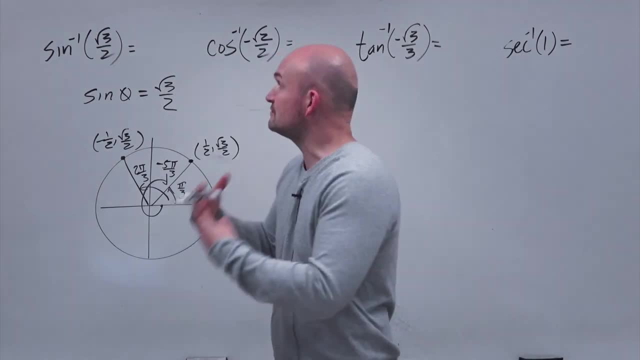 multiple solutions, And that's when we can try to evaluate an inverse function. Because if I'm trying to find what is the inverse function, what is the only angle that is going to satisfy, what is the only angle that's going to satisfy for the y-coordinate to be? 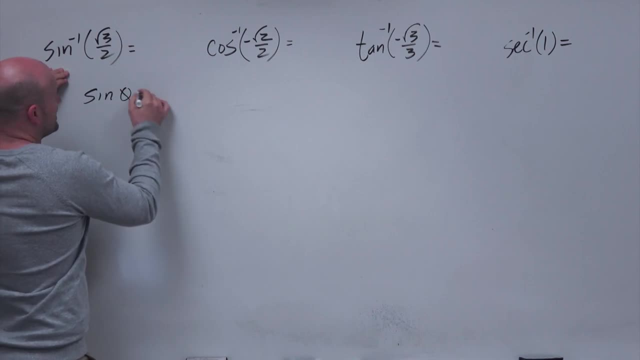 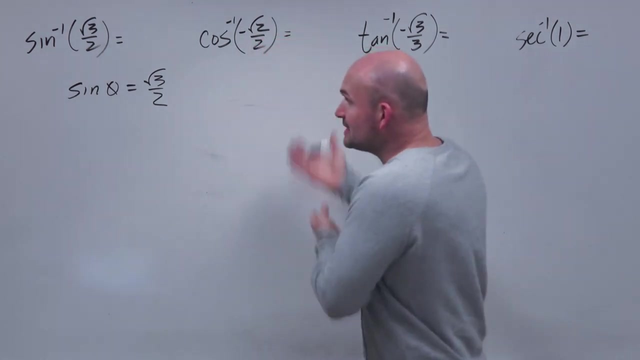 look at this as an equation. If I said the sine of theta is equal to the square root of three over two, right, what I'm saying is the sine of what angle is equal to square root of three over two? Now you could think of the square root of three over two as opposite over hypotenuse, but once. 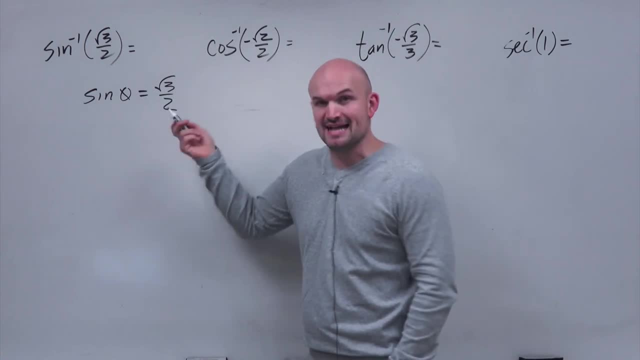 we've evaluated from the unit circle, we like to think of the sine as the y-coordinate of that point on the unit circle, because obviously those coordinate points are created from triangles. So if I'm thinking about this, I say, all right, well, when is the sine of theta equal to square? 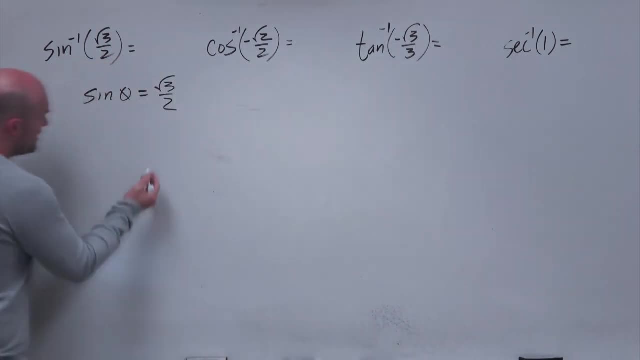 root of three over two right. So just thinking about this and we say, well, if we go ahead and take a look at the unit circle here, we recognize now that there's actually a point right here And we can say: all right, that point, that. 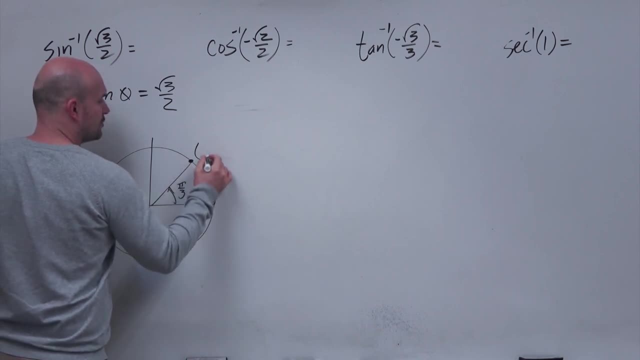 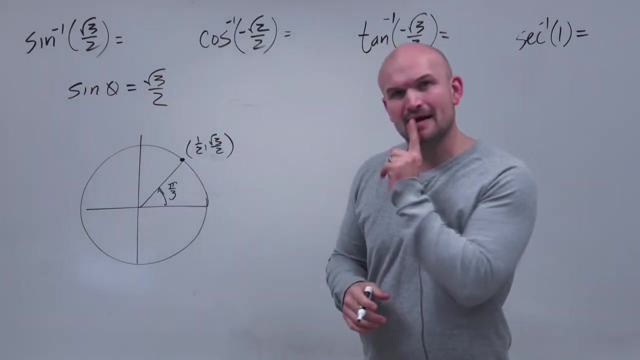 one's pretty easy. that is going to be pi over three, because this coordinate point is going to be one half comma, square root of three over two, right Done. But then we start to think we say, oh, wait a minute, I think there's more points. What about this? 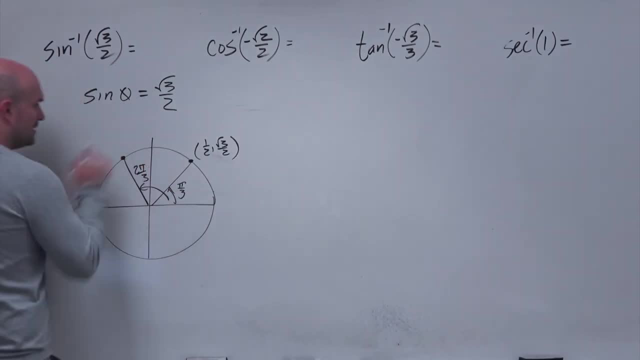 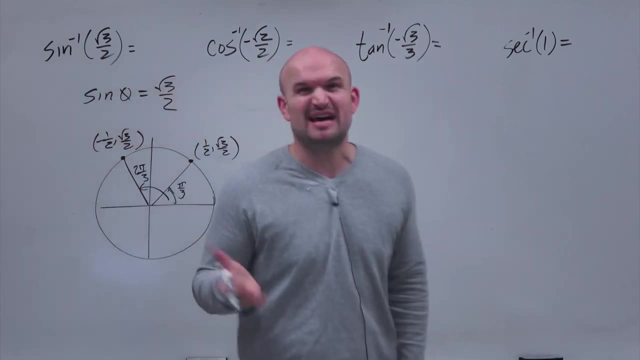 point over here, What about two pi over three? Because that point just has a negative x value but it still has a positive y value, And say, okay, well, we have two values, like we can have two answers, right. And then we say, well, wait a minute, what about negative five pi? 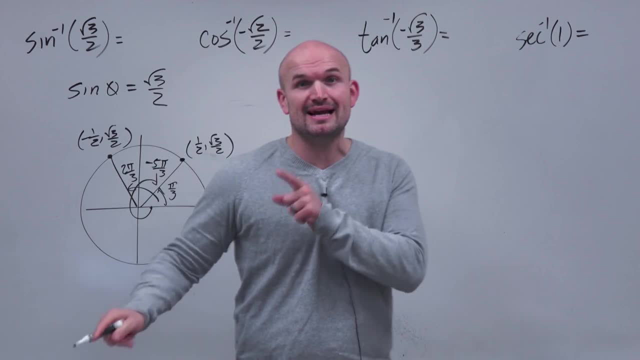 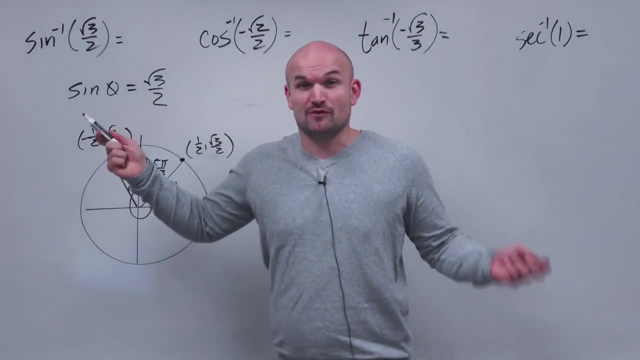 over three. Well, that works. And then we start going down coterminal angles and we recognize that we can keep on going around, and around and around the circle. So if we're not looking for one angle, we're actually looking for infinite many answers. So the 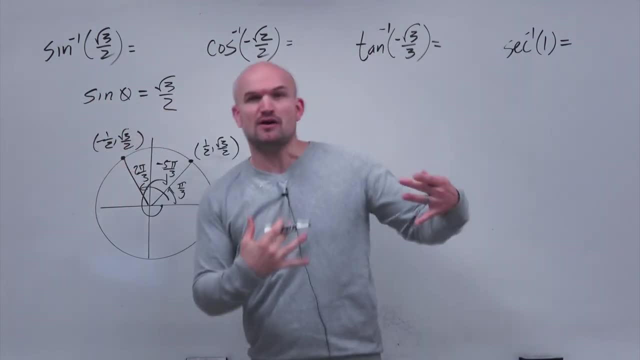 problem doesn't come back with this equation, because that makes sense for an equation We can solve. for an equation with multiple solutions. The problem comes into when we're dealing, when we're trying to evaluate the equation we can solve for an equation with 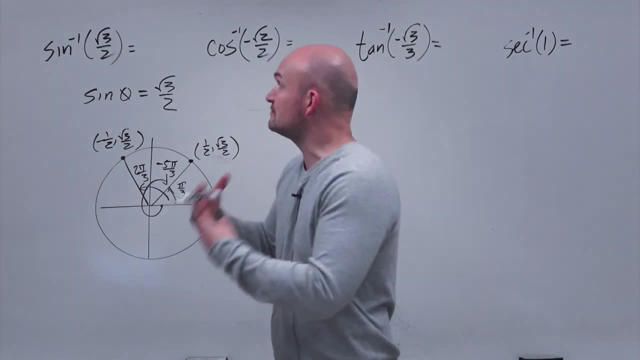 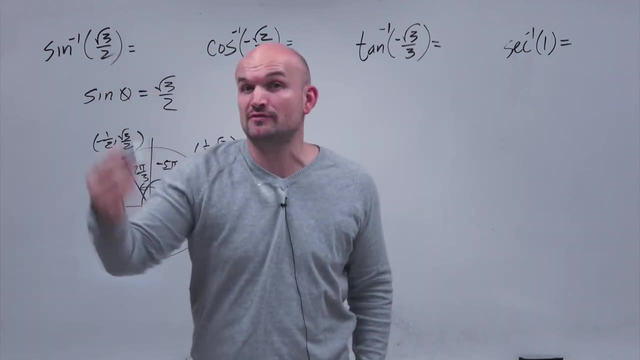 an inverse function. Because if I'm trying to find what is the inverse function, what is the only angle that is going to satisfy, what is the only angle that's going to satisfy for the y-coordinate to be square root of three over two? What we have to do is we have 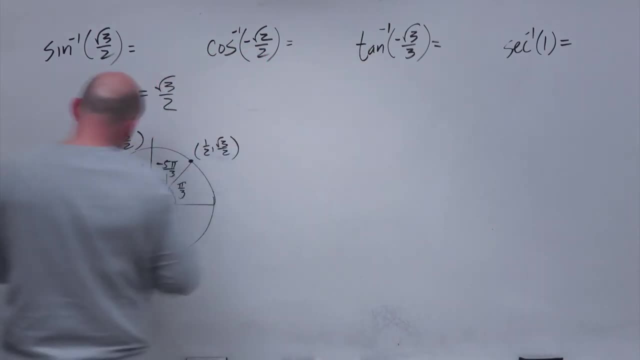 to restrict our original sine function And the restrictions that we use, that we teach in the class is the restrictions for sine is going to be between negative pi halves and pi halves. So now the question is a little bit different. I'm still asking myself the 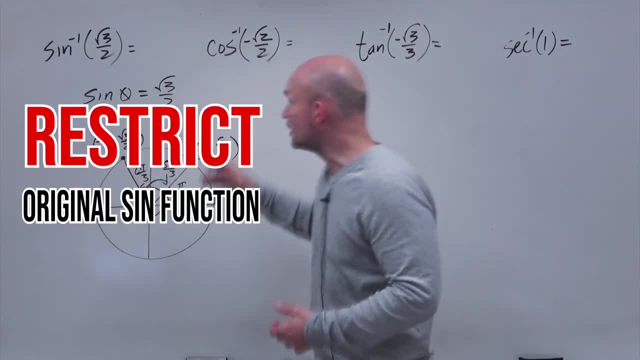 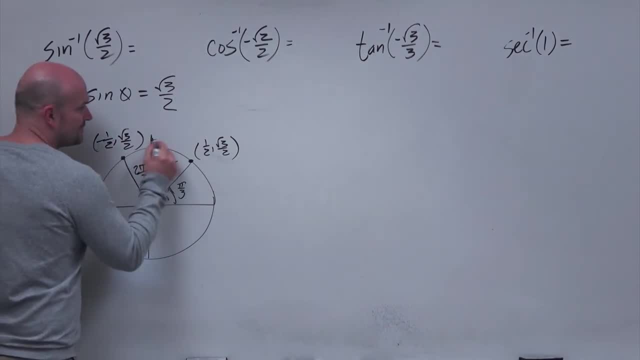 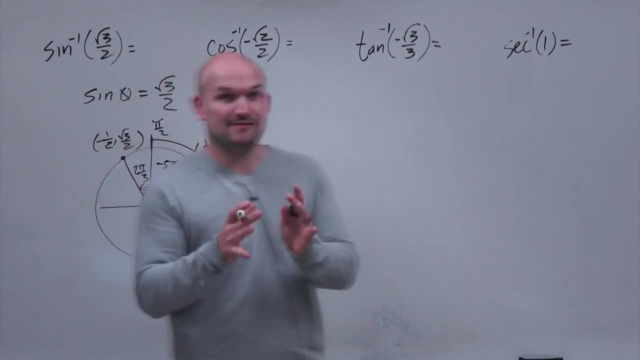 squared of three over two. What we have to do is we have to restrict our original sine function And the restrictions that we use. that we teach in the class is the restrictions, for sine is going to be between negative pi-halves and pi-halves. So now the question is a little. 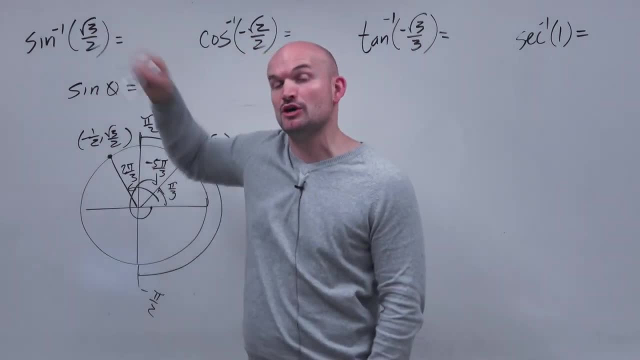 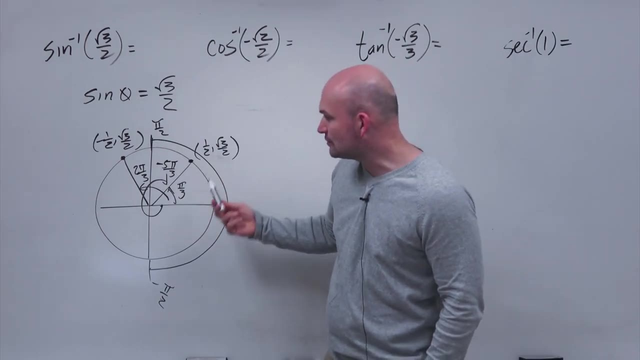 bit different. 007 angle gives me square root of 3 over 2. that matches the restriction for sine, which means my angle has to be between negative pi halves and pi halves. Well, the only angle that satisfies that is pi thirds or just pi over 3.. Now you might say: well, what about negative 5? 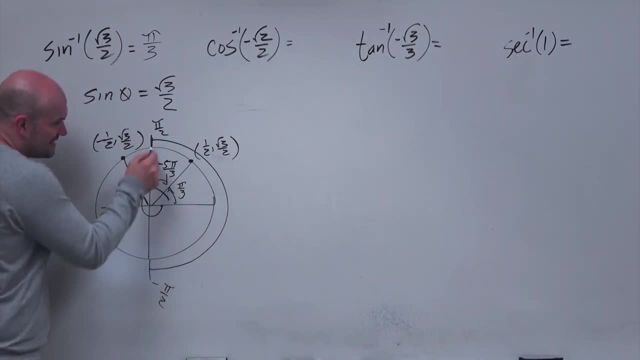 pi over 3?? Well, it's nice to kind of look at the graph, but since this is going outside of this restriction, so since this angle goes outside of the restriction, it's not going to be defined. So therefore, when you're looking for evaluating your inverse trigonometric 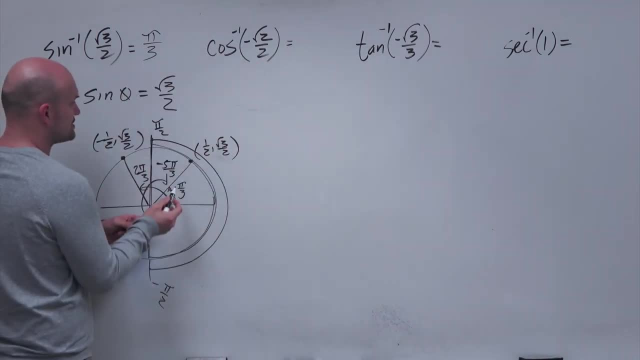 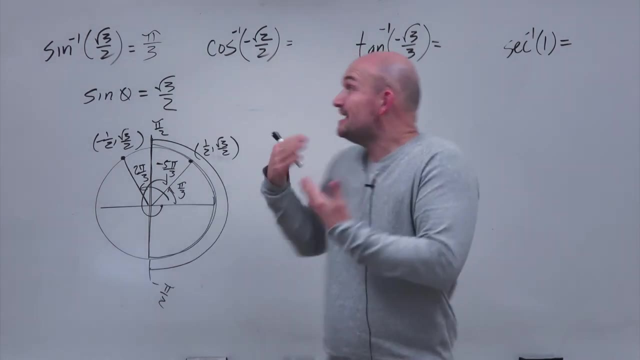 functions. your angle has to remain within the restrictions between negative pi halves and pi halves. Now let's go and take a look at another example for cosine. Now, again, if we're doing the inverse cosine, we can only have one answer: It's a function, You. 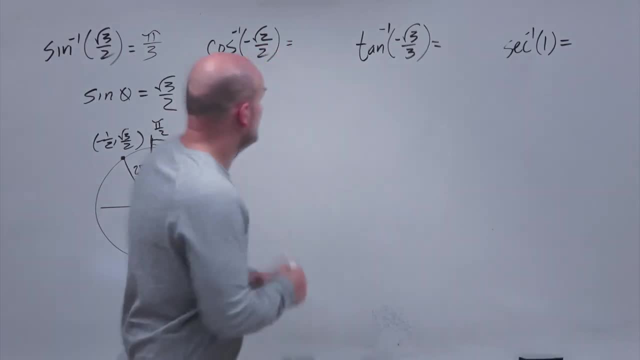 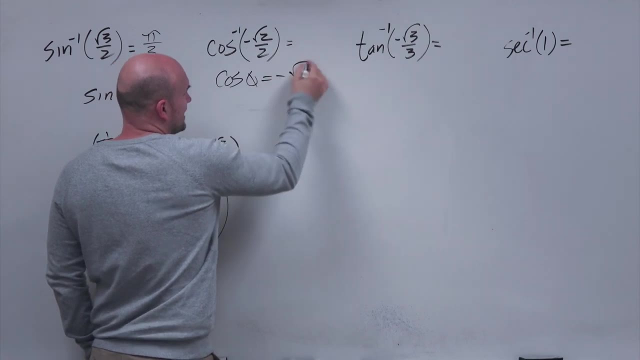 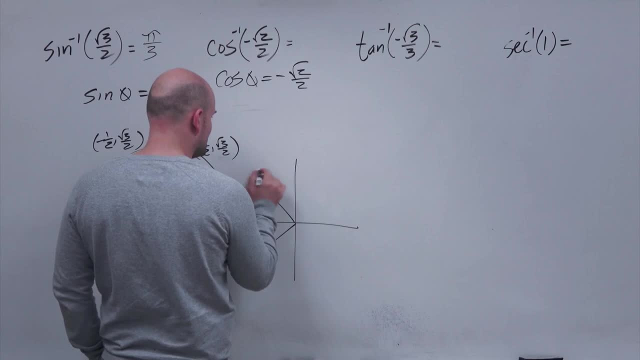 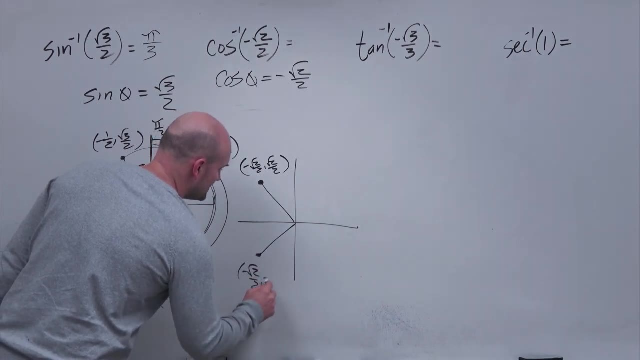 and I think over here and down here. So this point, you know, this would be a negative square root of 2 over 2, comma, square root of 2 over 2.. And this point would be negative square root of 2 over 2, comma, negative square root of 2.. And you say: well, what are these? 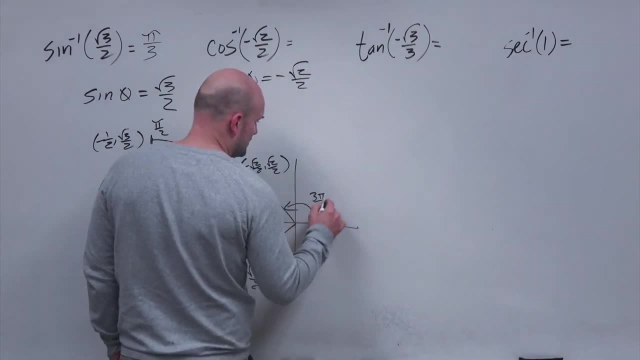 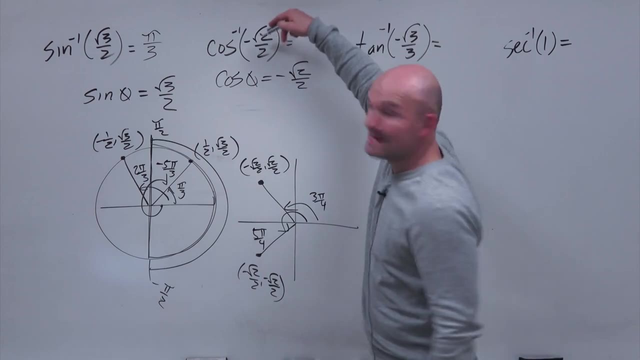 two points right, We have. this point's going to be a 3 pi over 4. And this point is going to be a 5 pi over 4.. Now again, we can't have, for one answer, given us two answers. 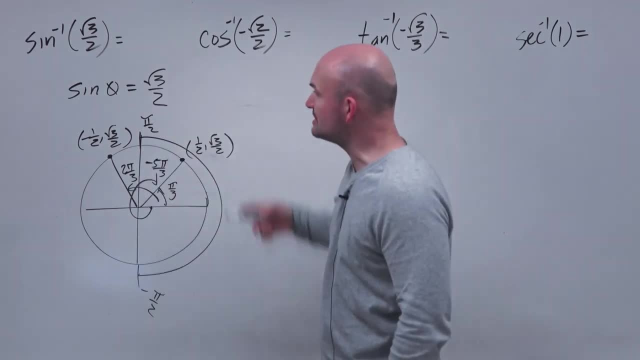 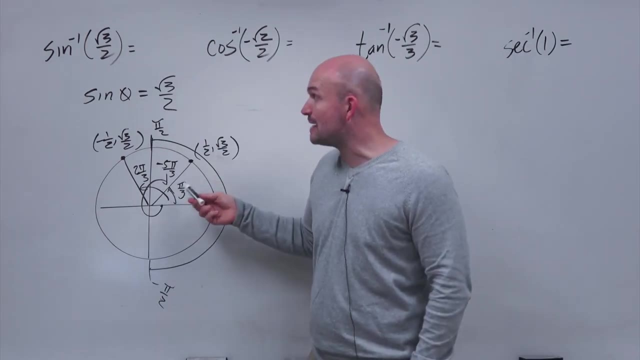 question: how do I know that my angle is going to be between negative pi halves and pi halves? Well, the only angle that satisfies that is pi thirds or just pi over three. Now you might say, well, what about negative pi over three? Well, it's nice to kind of 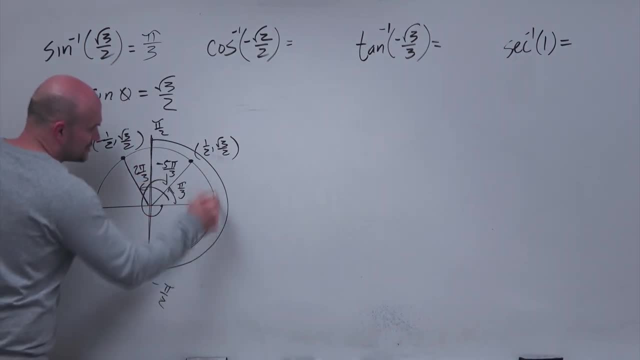 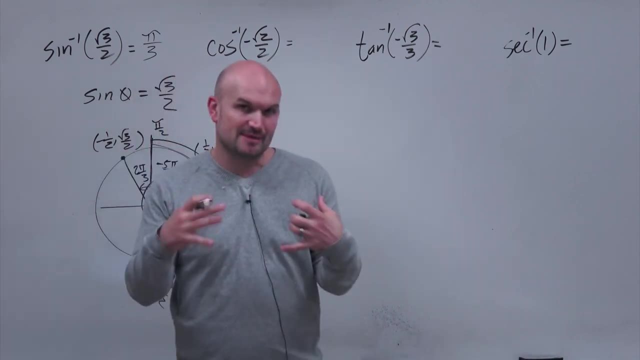 look at the graph. but since this is going outside of this restriction, so since this angle goes outside of the restriction, it's not going to be defined. So therefore, when you're looking for evaluating your inverse trigonometric functions, your angle has to. 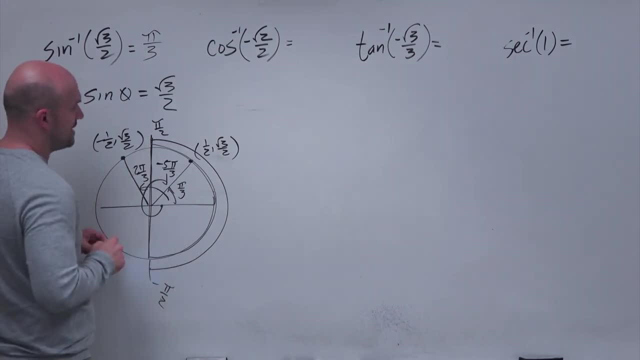 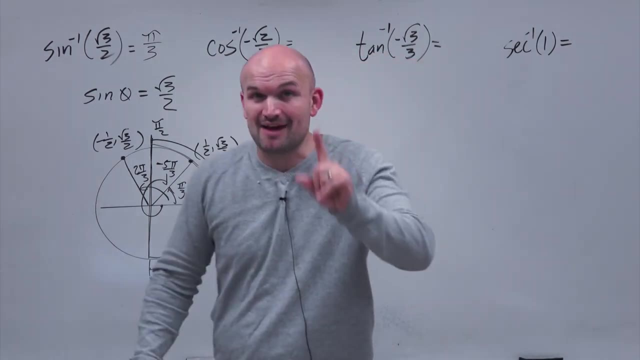 remain within the restrictions between negative pi halves and pi halves. Now let's go and take a look at another example for cosine. Now again, if we're doing the inverse cosine, we can only have one answer. It's a function. You plug something in you. 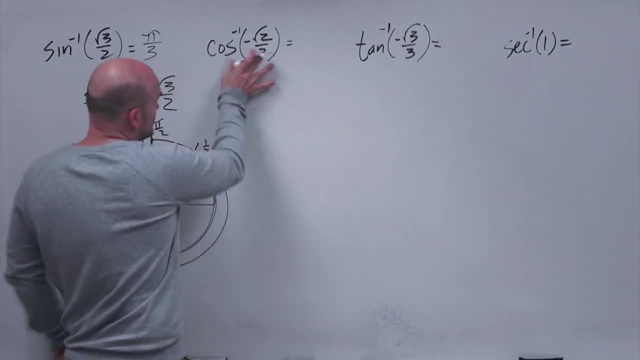 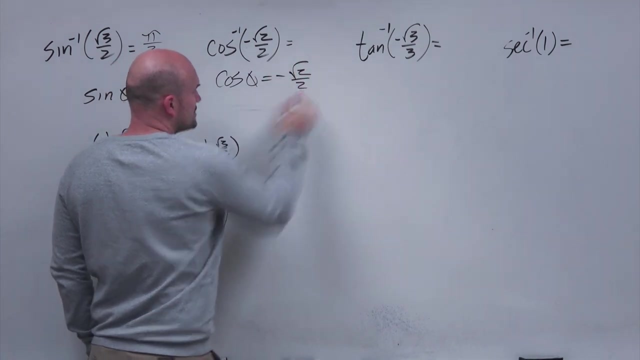 get something out. You can't have two answers. But when we look at the unit circle and we say what are the x values- because basically we're saying cosine of what angle is equal to a negative square root of two over two- Well, immediately in my brain I think of 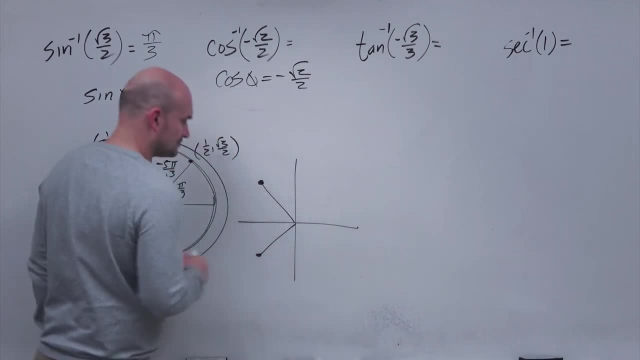 these two answers, I think, over here and down here. So this point, this would be a negative square root of two over two comma, square root of two over two, And this point would be negative. square root of two over two comma negative. 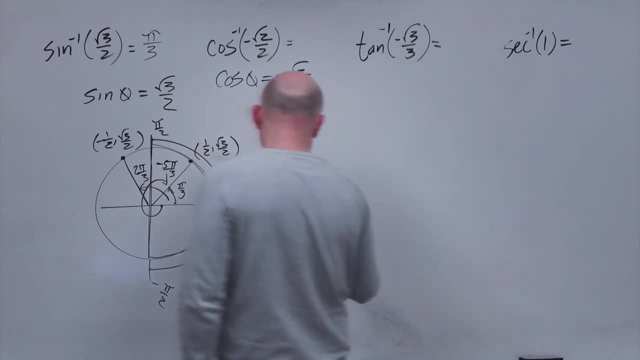 square root of two And then say, well, what are these two points? We have this point's going to be a three pi over four, And this point is going to be a five pi over four. Now again, we can't have, for one answer, given us two answers. So we have to say well, which? 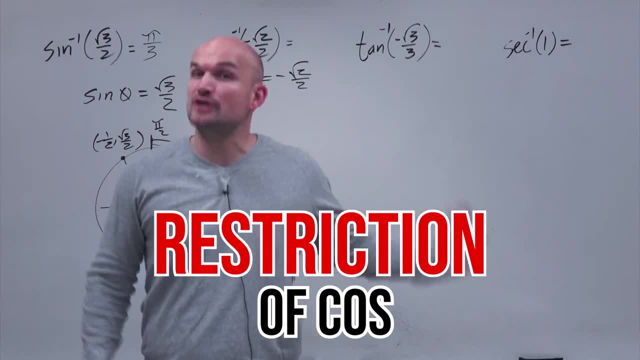 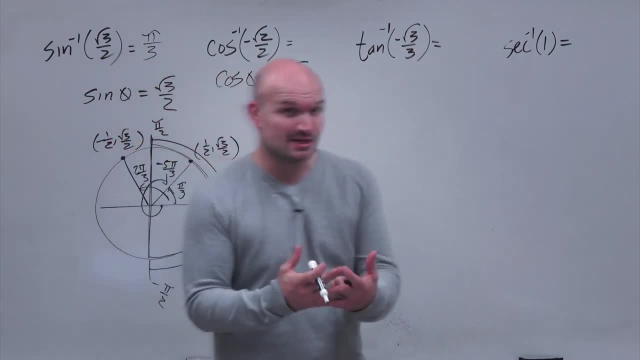 one, is it? So again, they have to follow the restrictions of cosine, And we restrict the sine function between zero and pi. So therefore, the only answer, when I'm trying to find the inverse cosine of negative square root of two over two, your answer, your angle, has to be: 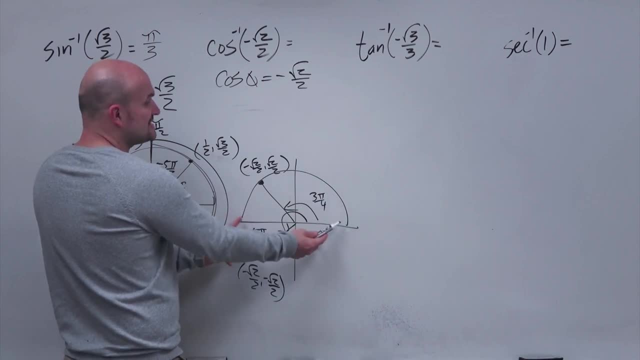 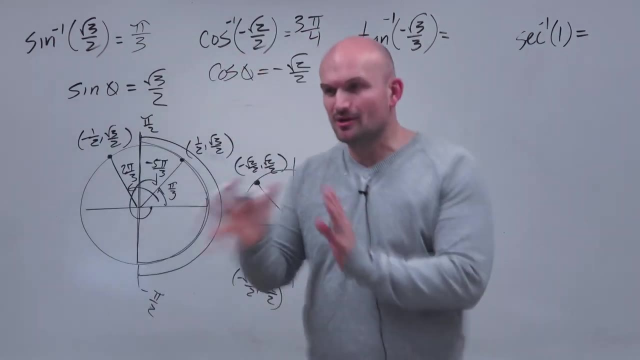 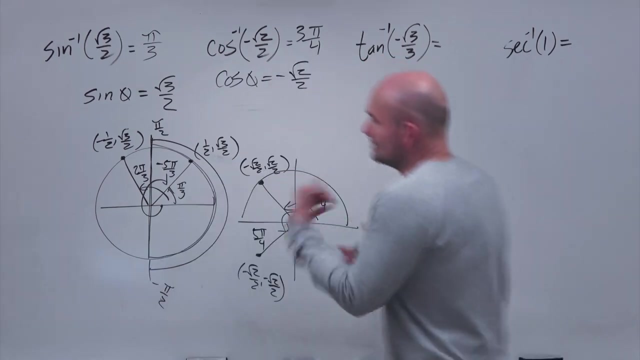 between zero and pi. So the only angle here that satisfies that restriction, as well as our function, is going to be three pi over four. So it gets a little bit easy when you start looking at knowing the restrictions for sine, knowing the restrictions for cosine, because all you're really doing is looking at the 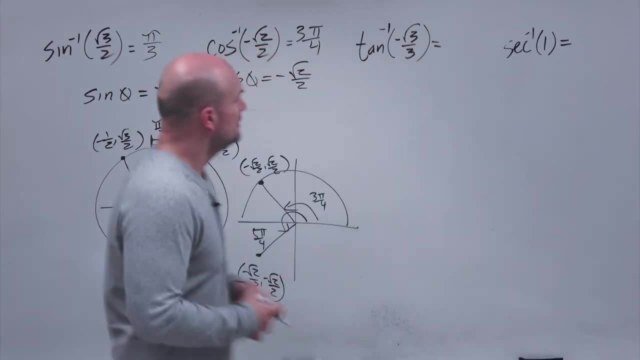 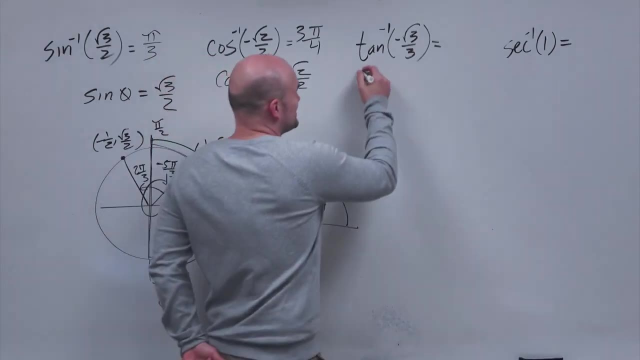 angles on the unit circle that match those restrictions. Then we get into tangent And it's like ah, tangent, crap. I don't know tangent Because, remember, tangent is your y over your x, So you've got to think. all right, I know this. 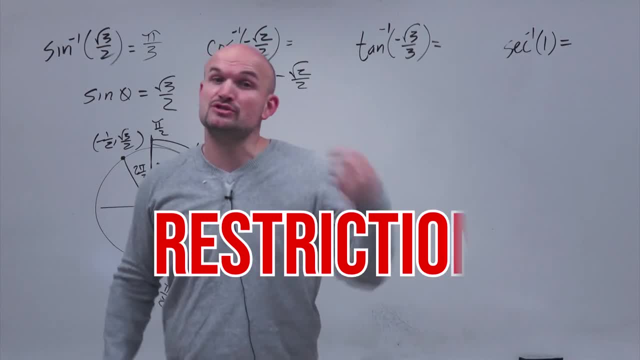 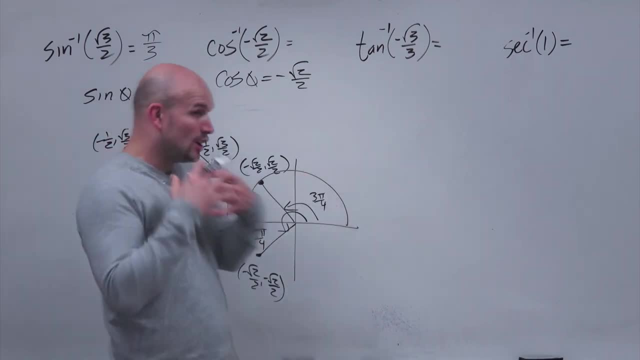 So we have to say: well, which one is it? So again, they have to follow the restrictions of sine, And we restrict the cosine function between 0 and pi. So therefore, the only answer, when I'm trying to find the inverse cosine of negative square root of 2 over 2, your. 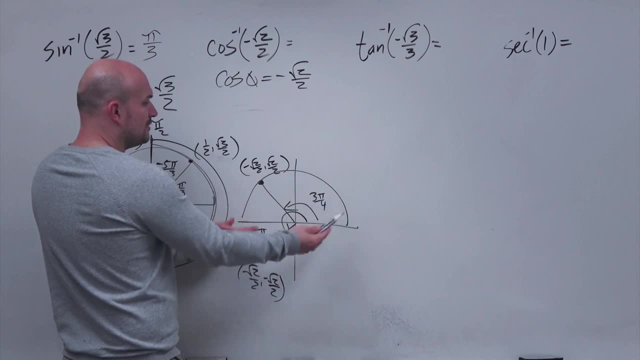 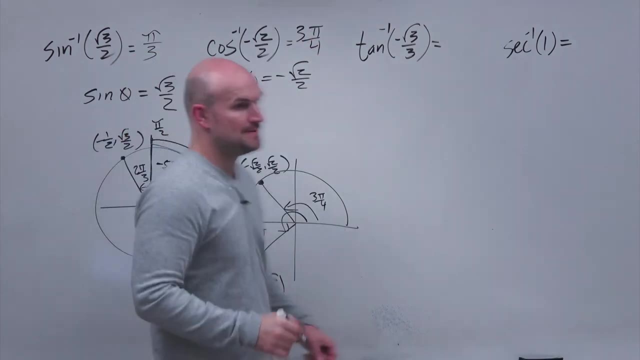 answer. your angle has to be between 0 and pi. So the only angle here that satisfies that restriction, as well as our function, is going to be 3 pi over 4, OK, So it gets a little bit easy when you start looking at knowing the restrictions for sine knowing. 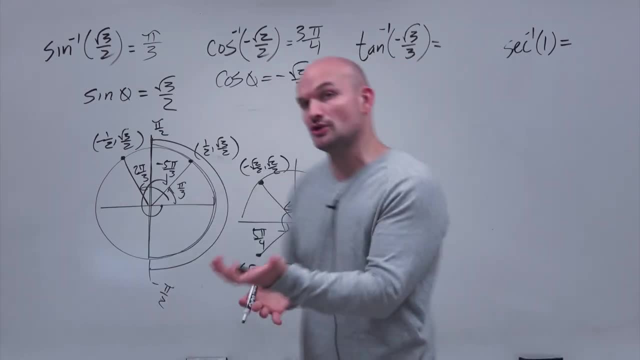 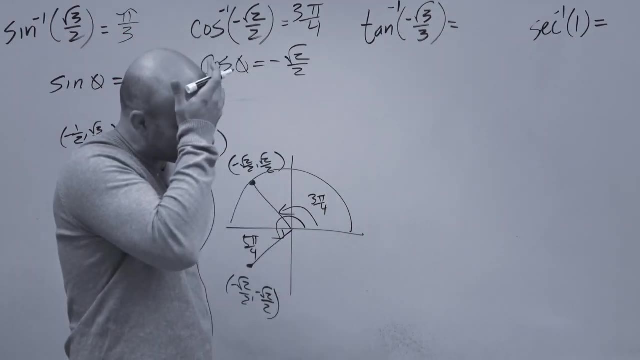 the restrictions for cosine, because all you're really doing is looking at the angles on the table that match those restrictions. OK, Then we get into tangent And it's like: ah, tangent, Crap. I don't know tangent Because. 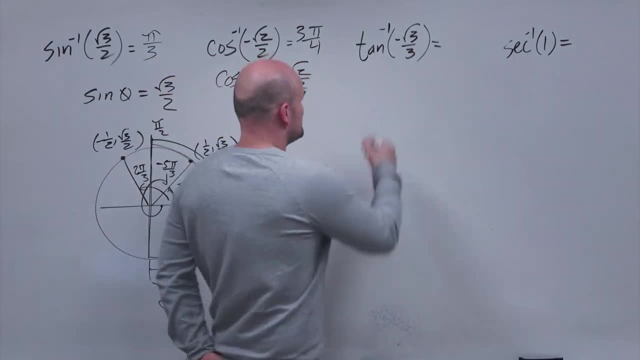 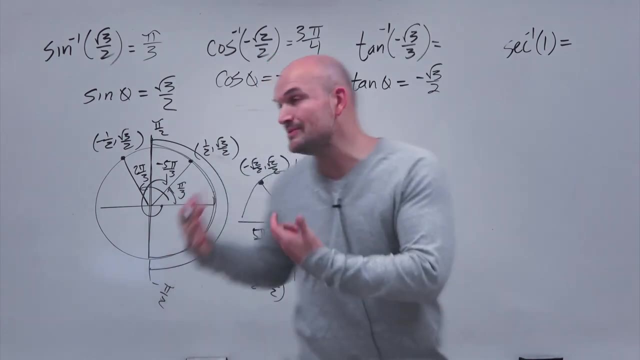 remember, tangent is your y over your x, right? So you've got to think: all right, I know this Tangent of what angle is going to equal negative square root of 3 over 2? Now it's nice when you have the x or the y coordinates, because you can just kind of look at your 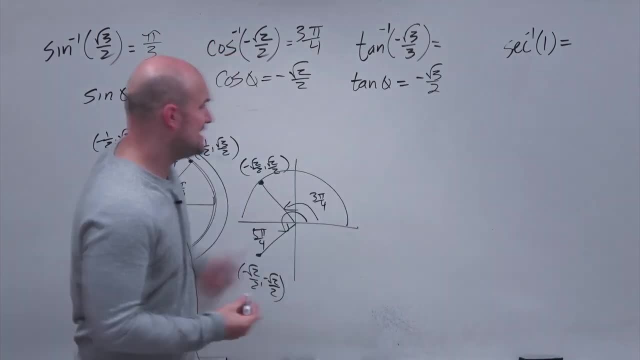 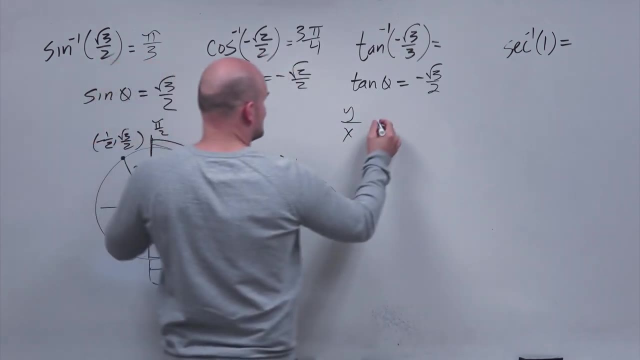 unit circle and say, oh, that's the angle or that's that point. But when you have tangent, remember this is y over x. So we're trying to think: all right, If you look at a coordinate point, is that going to be square root of 3 over 2 over 1? 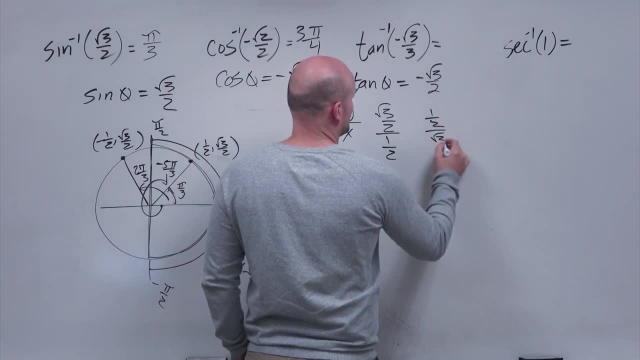 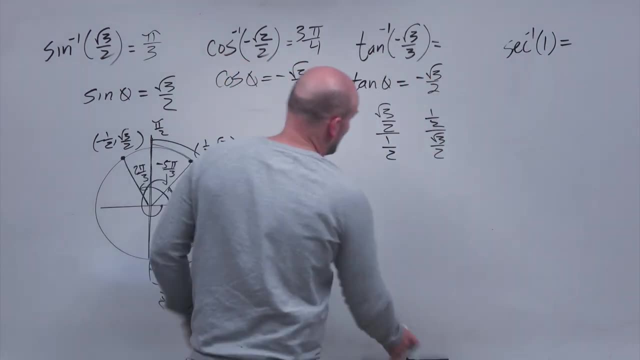 half, Or is it 1 half over square root of 3 over 2?? And so we have to remember which one of these is going to give us square root of 3 over 2.. And hopefully, with your practice throughout the unit circle, you recognize that this is going to simplify to the square. 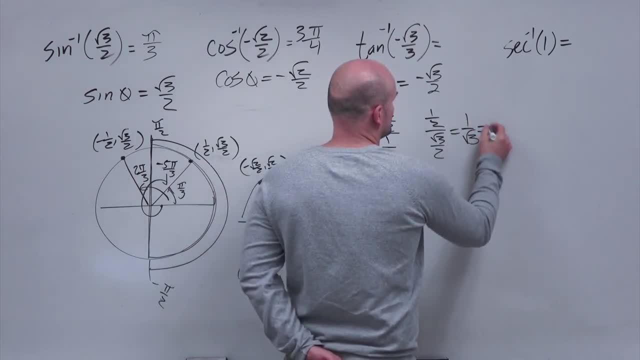 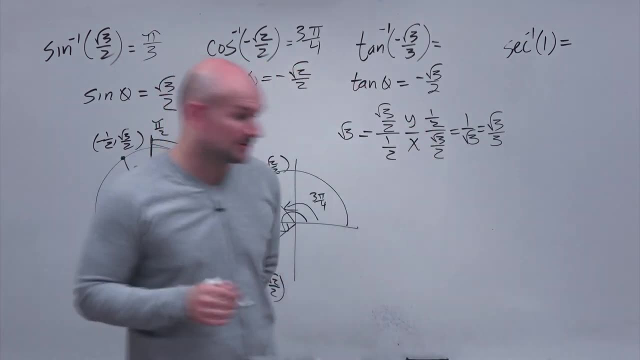 root of 3.. And this simplifies to 1 over the square root of 3, which is square root of 3 over 3.. So therefore, that means this is my y coordinate And this is my x coordinate. So if this is my y coordinate and this is my x coordinate, I need to be able to figure. 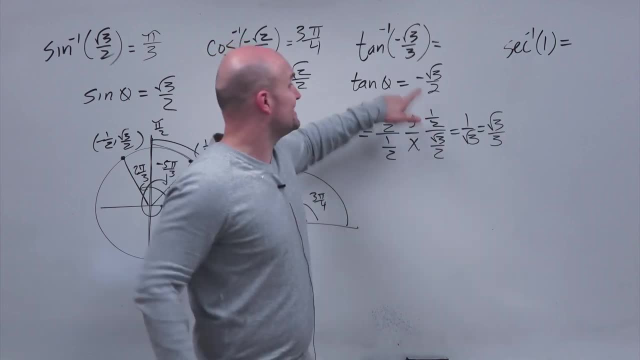 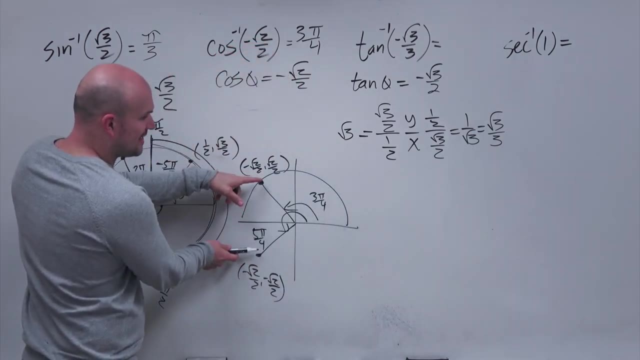 out all right. well, where in the unit circle is this going to be y? this is x, but them being negative. So immediately once I see tangent's negative, I think: OK, just like how I knew cosine was negative to the left of the y-axis, sine was positive above the x-axis. I know that tangent. 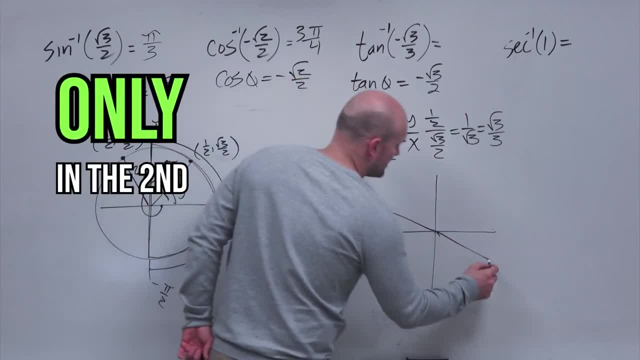 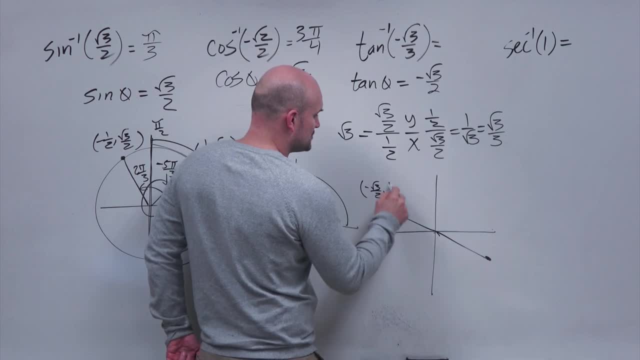 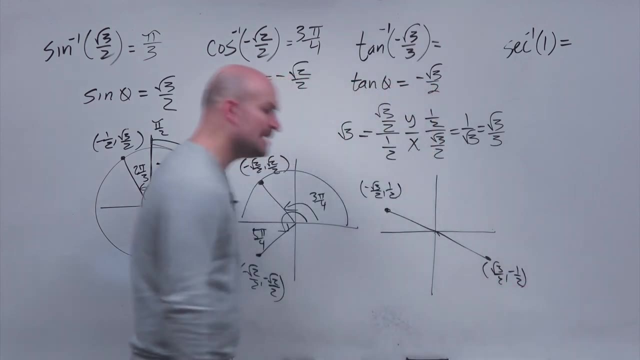 is negative only in the second and the fourth quadrant And if y is 1 half and x is square root of 3 over 2, the only points that make sense is negative square root of 3 over 2, comma 1 half, as well as positive square root of 3 over 2, comma negative 1 half. 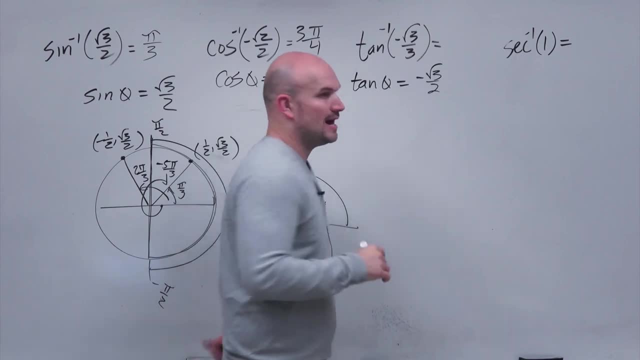 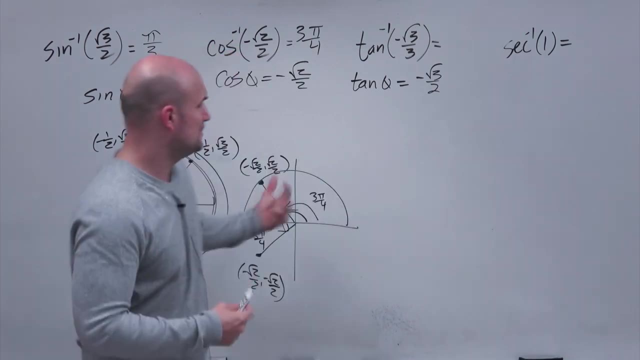 Tangent of what angle is going to equal negative square root of three over two. Now it's nice when you have the x or the y coordinates because you can just kind of look at your unit circle and say, oh, that's the angle or that's that point. But when you have tangent, 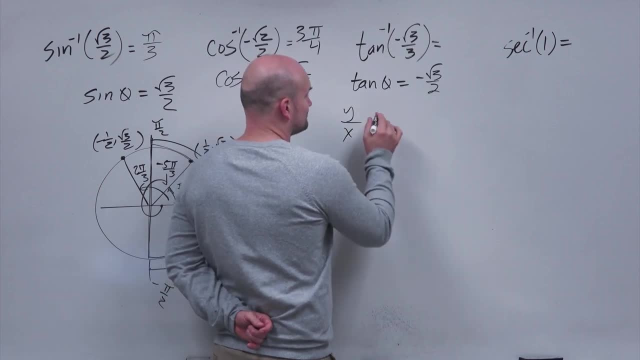 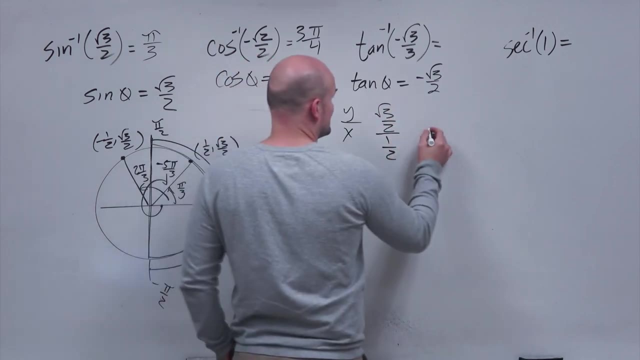 remember this is y over x. So we're trying to think, all right, well, if you look at a square root of three over two, is that going to be square root of three over two over one half, Or is it one half over square root of three over two? And so we have to remember. 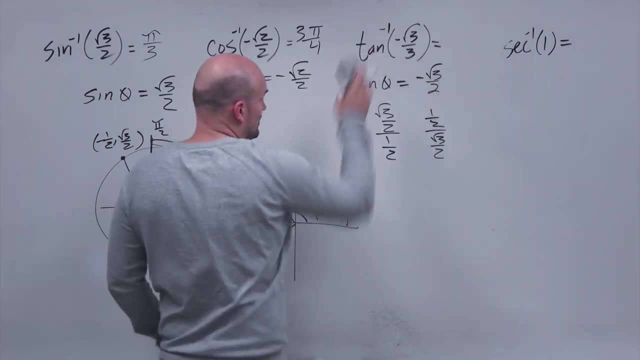 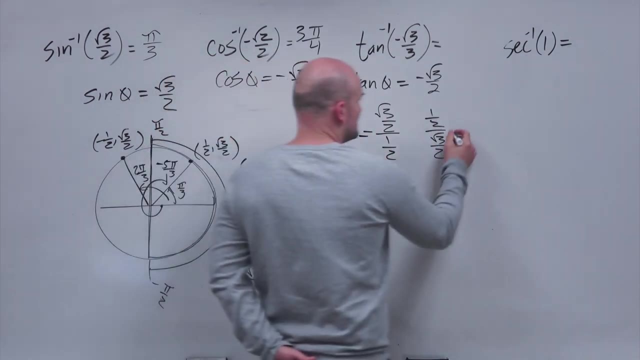 which one of these is going to give us square root of three over two And hopefully, with your practice throughout the unit circle, you recognize that this is going to simplify to the square root of three And this simplifies to one over the square root of three, which 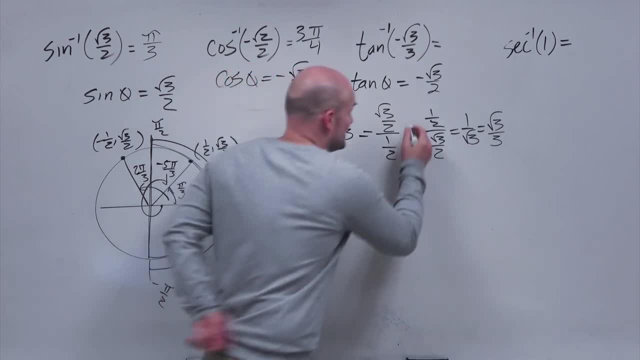 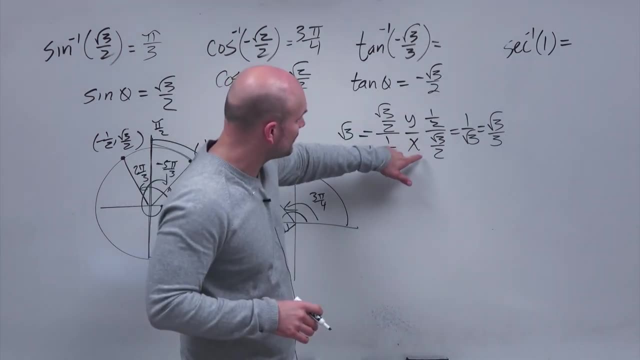 is square root of three over three. So therefore, that means this is my y coordinate and this is my x coordinate. OK, So if this is my y coordinate and this is my x coordinate, I need to be able to figure out all right. well, where on the unit circle is this going to be y? this is x, but them. 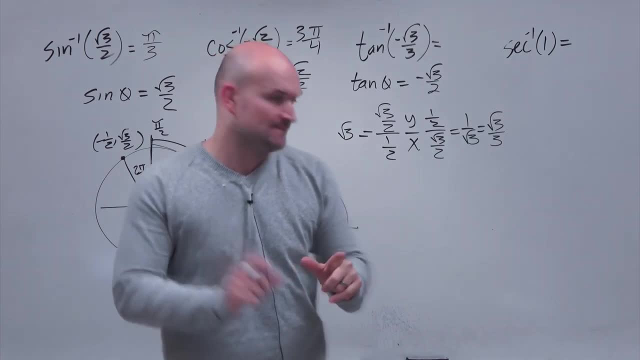 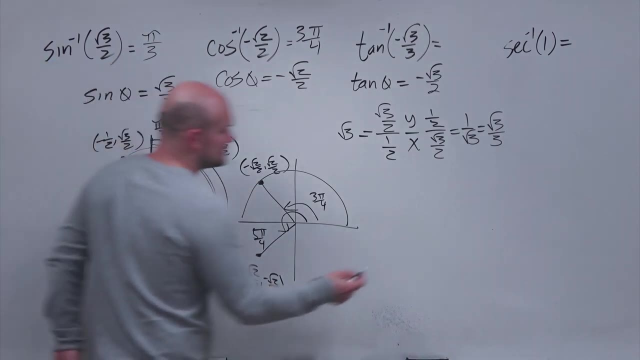 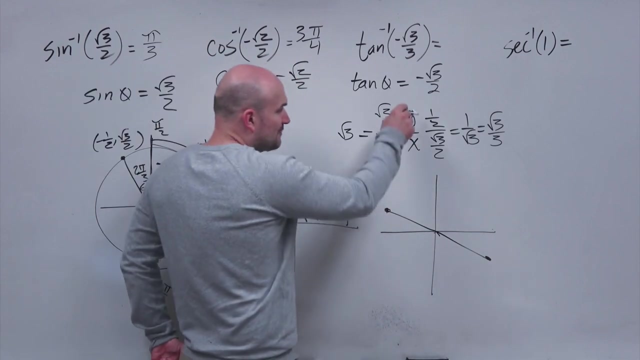 being negative. So immediately, once I see tangent's negative, I think: OK, just like how I knew cosine was negative to the left of the y-axis, sine was positive above the x-axis, I know that tangent is negative only in the second and the fourth quadrant And 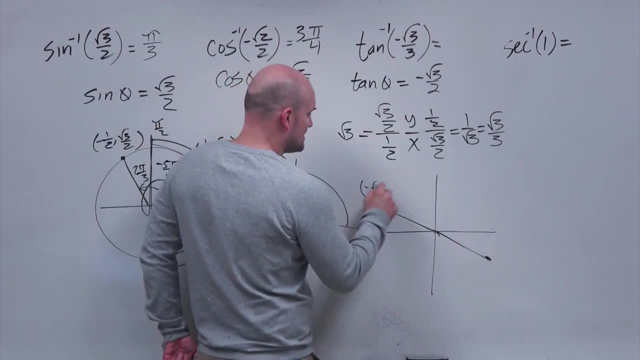 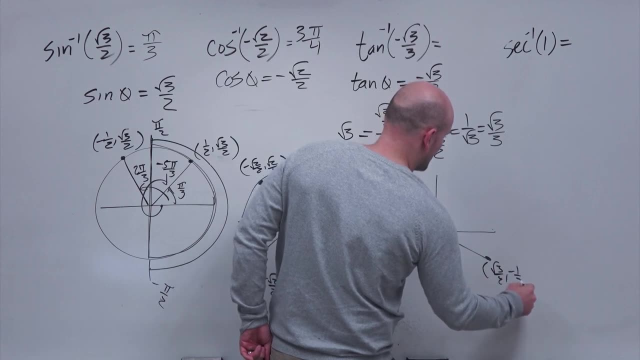 if y is one half and x is square root of three over two, the only points that make sense is negative square root of three over two, comma one half, as well as positive square root of three over two, comma negative one half. Now, when we get into cotangent, the restrictions for our tangent function are going to be the 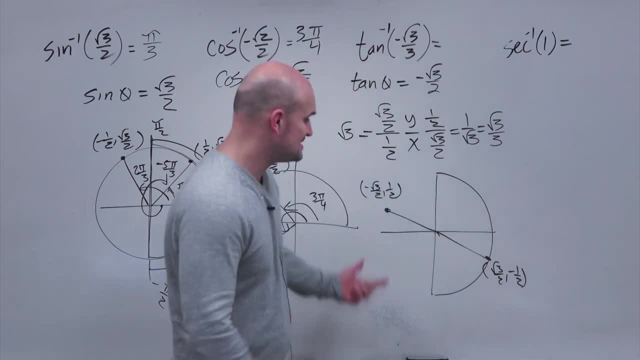 same as the restrictions for the sine function. That means the angles need to be between negative pi halves and pi halves. So now what I got to do is be able to find an angle that's going to satisfy the solution, And a lot of students will go from here and they say, OK, well, 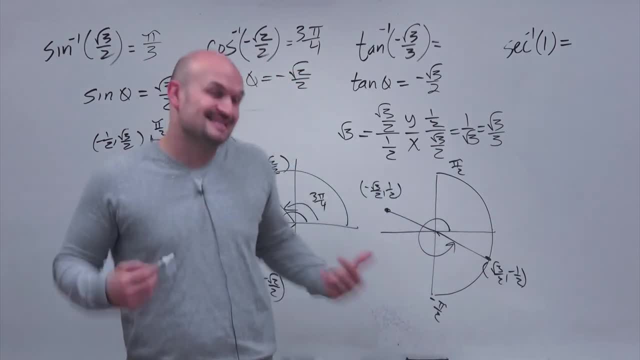 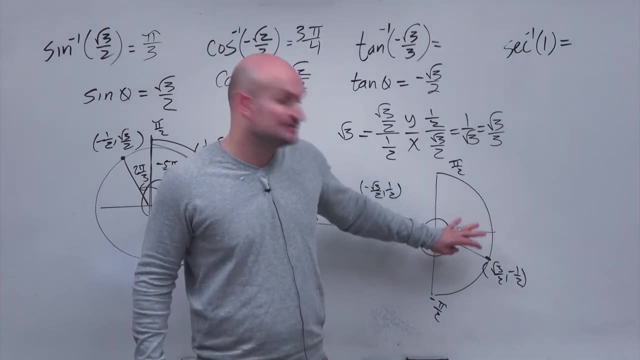 it can't be this one, It'll be right there. But again, the same thing is going on. We cannot go outside of our restriction. We have to have an angle that is going to maintain within the restriction of our inverse function. So therefore, instead of going outside, instead of going 11 pi over, 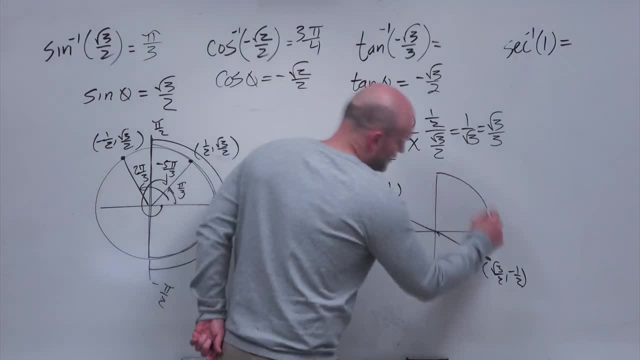 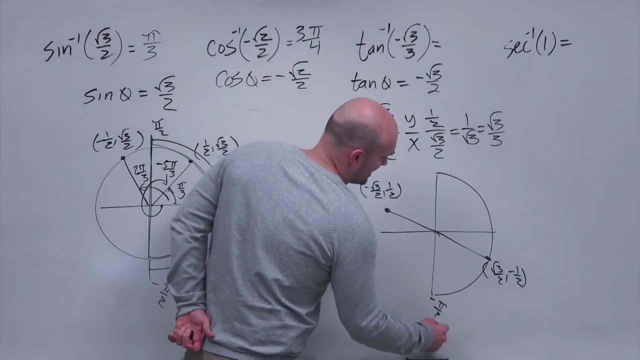 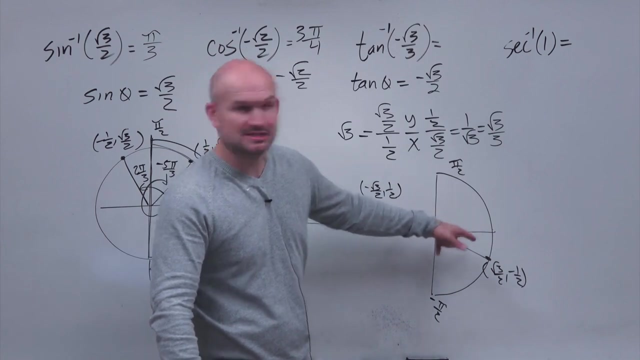 Now, when we get into tangent, the restrictions for our tangent function are going to be the same as the restrictions for the sine function. That means the angles need to be between negative pi halves and pi halves. So now what I've got to do is be able to find an angle that's going to satisfy the solution. 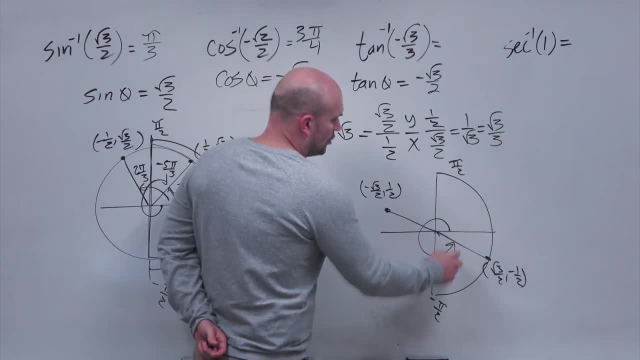 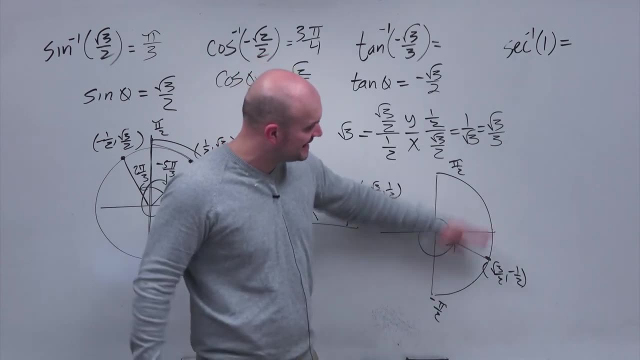 And a lot of students will go from here And they say, OK, well, it can't be this one, So it'll be right there. But again the same thing is going on. We cannot go outside of our restriction. We have to have an angle that is going to maintain. 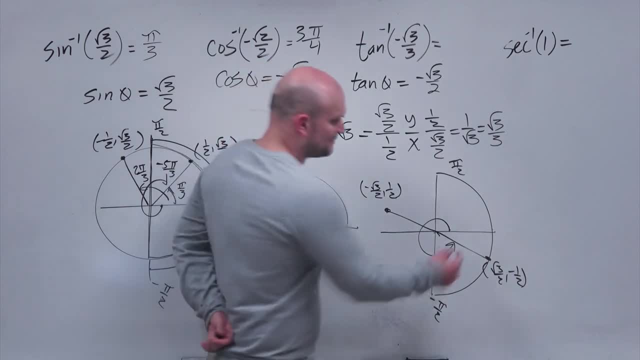 within the restriction of our inverse function. So therefore, instead of going outside, instead of going 11 pi over 6, we're going to have to go down in the negative direction, And that's why this answer is negative pi over 6.. So it's very important to understand. 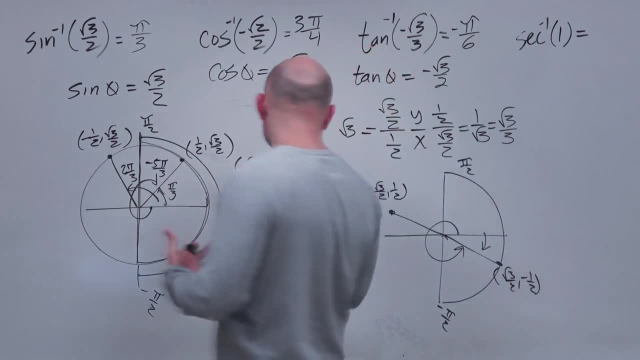 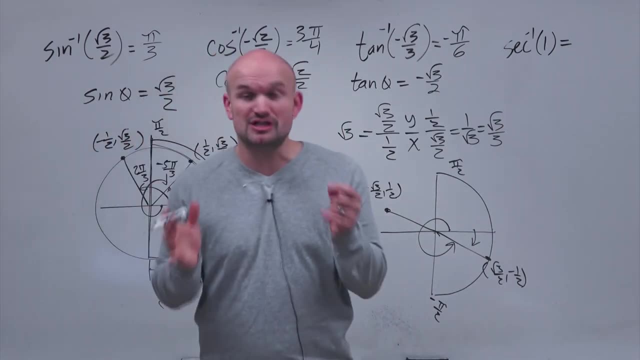 the stick within those restrictions. And again, the reason why we have the restrictions I don't even think I mentioned. I didn't want to go way down into that rabbit hole, But again, we have the restrictions. So therefore our function is going to be 1 to 1.. 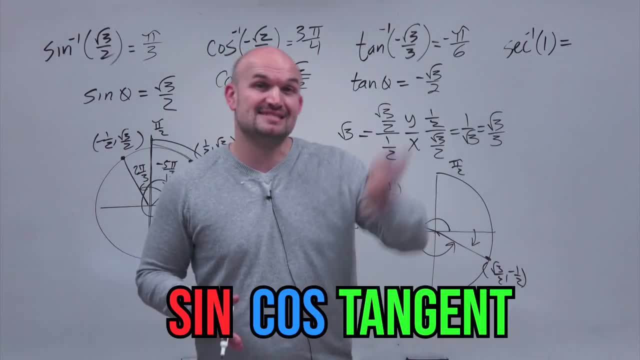 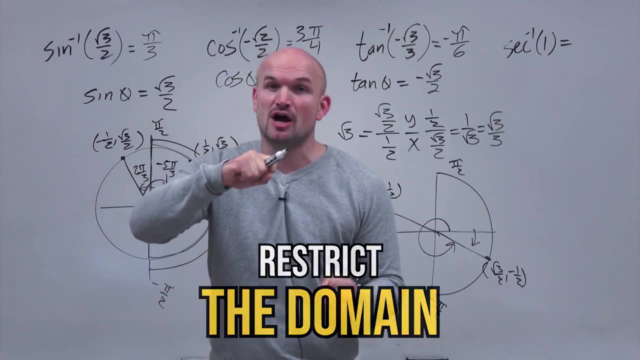 Because if we didn't have the restrictions, as you notice that sine and cosine, as well as tangent, they repeat And they fail the horizontal line test. They're not 1 to 1 functions. So what we do is we restrict the domain of our trigonometric functions. So therefore, 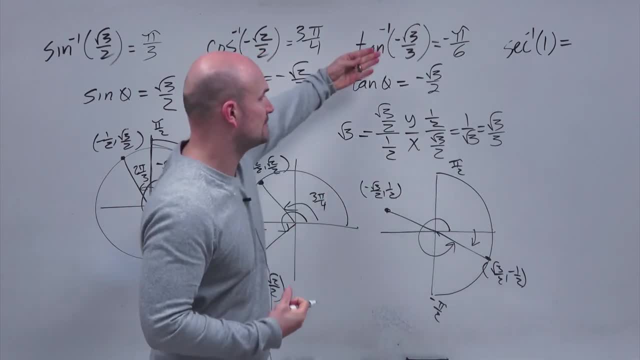 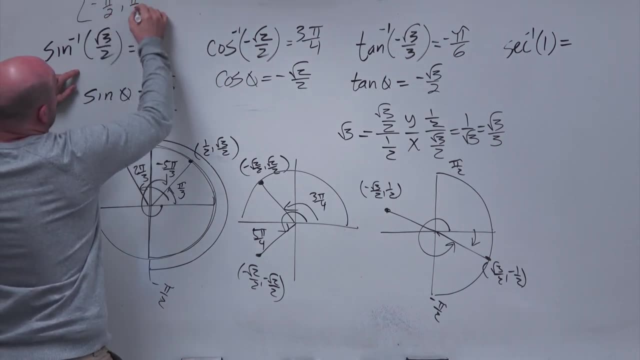 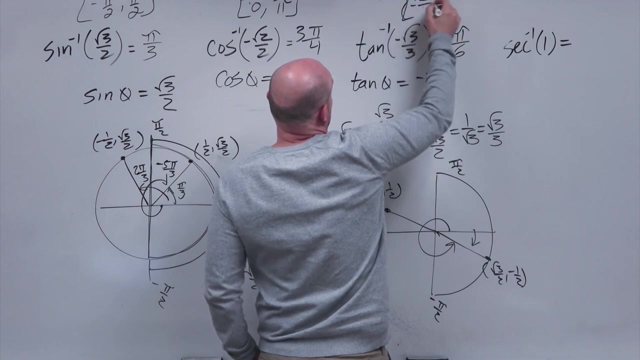 we can find the inverse or that the inverse is invertible And therefore we can restrict them. So the restrictions that we use for sine is going to be for negative pi halves to pi halves. For cosine it's going to be 0 to pi And tangent is negative pi halves. 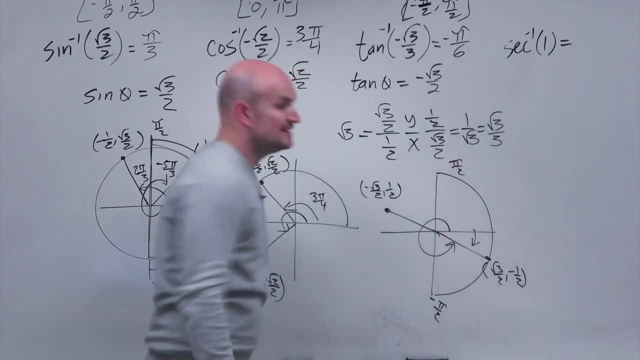 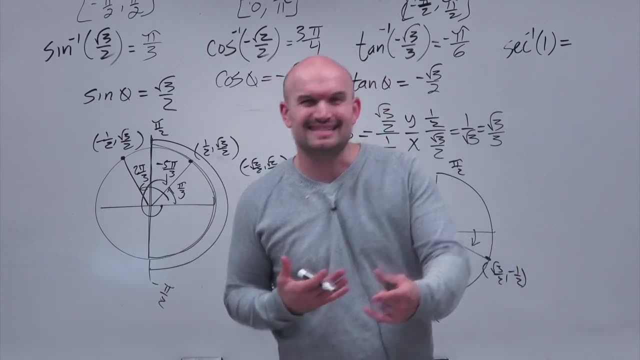 to pi halves. Okay. Now the last one I want to bring up is secant, And a lot of times when we're thinking of secant, sometimes it gets confusing. It's like, well, again, secant is that the inverse? A lot of students will mix up secant with the inverse, or the 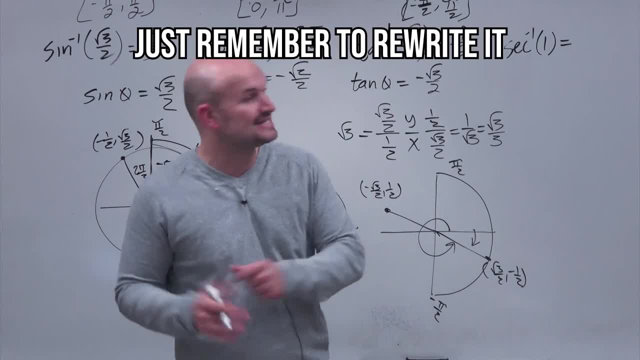 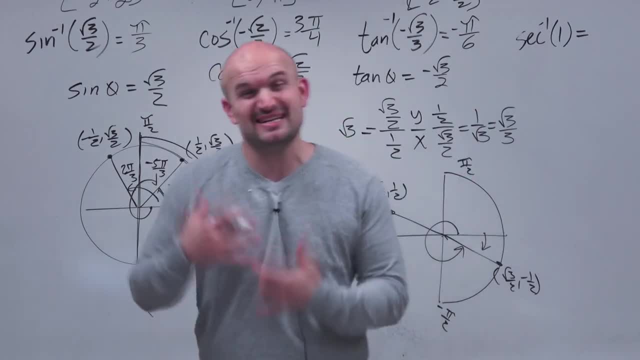 reciprocal. And again, my advice to you is: just remember to rewrite it as a equation and then use it in terms of cosine, Because we don't have in my notes. in my class we didn't talk about the restrictions of secant and looking at the graphs. We just looked at the graphs of these three. 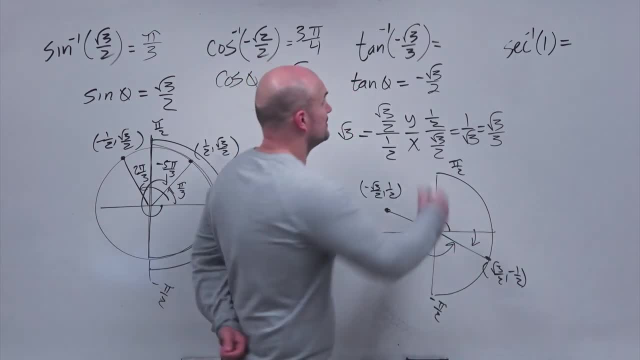 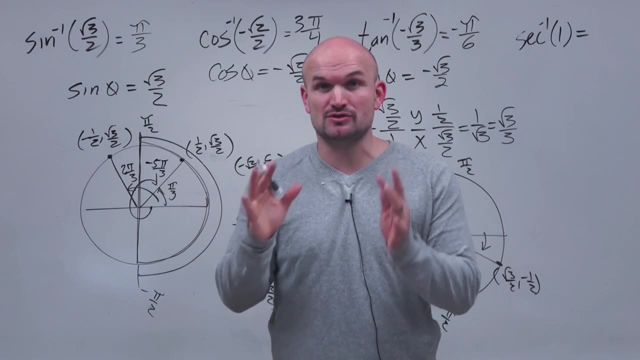 6,. we're going to have to go down in the negative direction And that's why this answer is negative: pi over 6.. OK, so it's very important to understand the stick within those restrictions And, again, the reason why we have the restrictions I don't even think I mentioned. I didn't want. 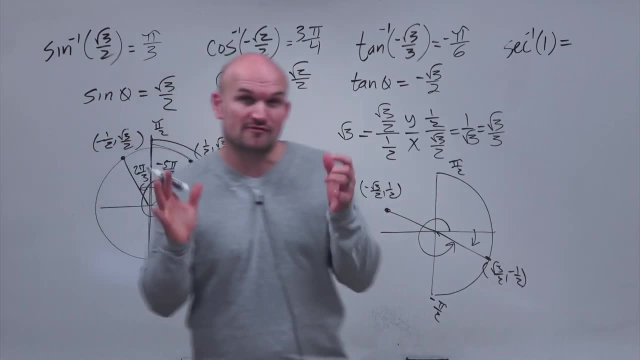 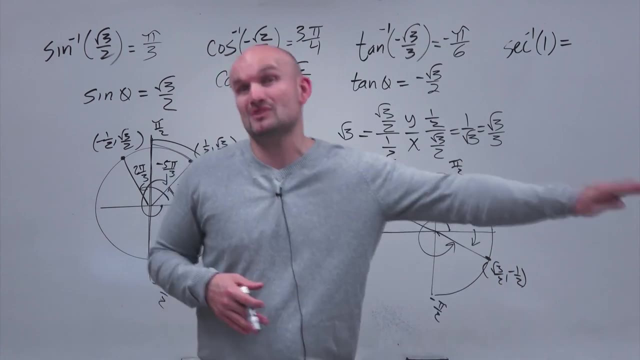 to go down into that rabbit hole. But again, we have the restrictions. So therefore our function is going to be one to one, Because if we didn't have the restrictions, as you notice that sine and cosine, as well as tangent, they repeat And they fail the horizontal. 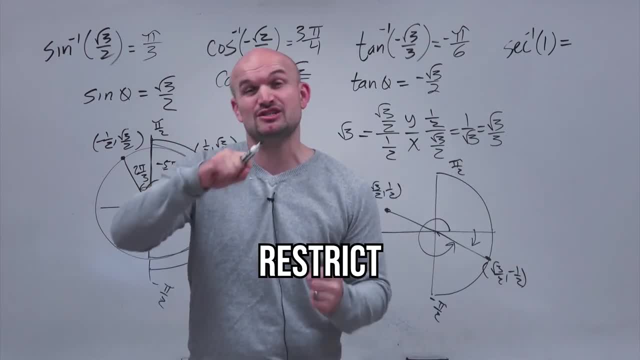 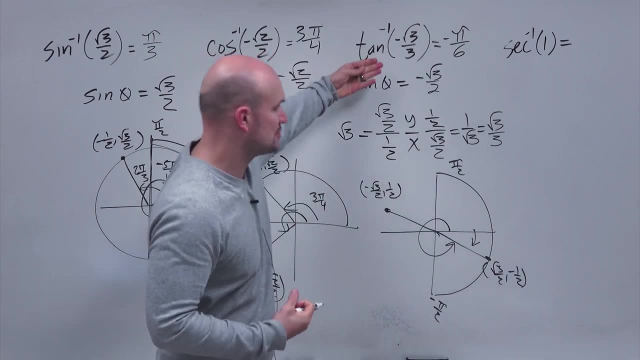 line test. They're not one to one functions. So what we do is we restrict the domain of our trigonometric functions. So therefore we can find the inverse, or that the inverse is invertible, And therefore we can restrict them. 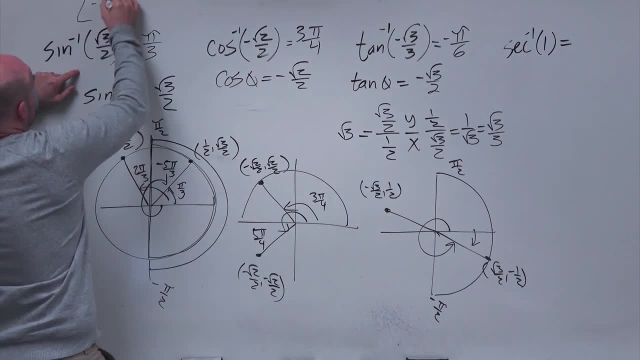 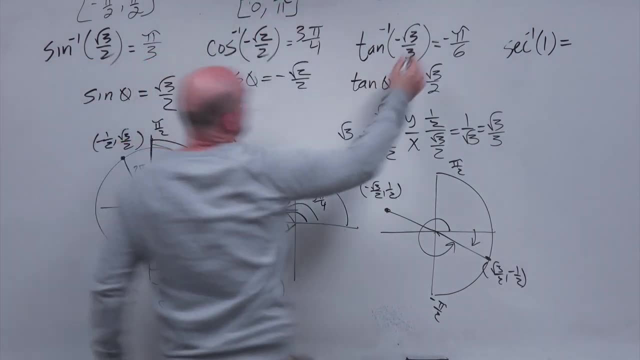 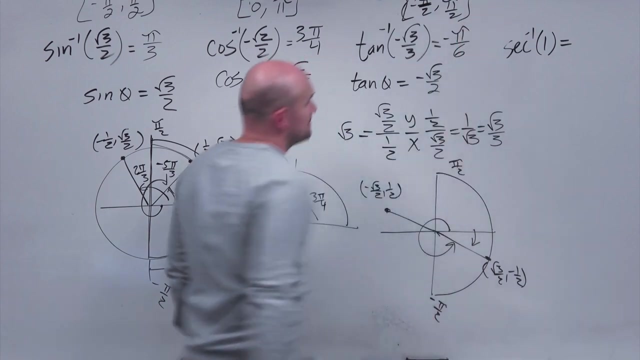 So the restrictions that we use for sine is going to be from negative pi halves to pi halves, Sine is going to be 0 to pi And tangent is negative pi halves to pi halves. OK, now the last one I want to bring up is secant, And a lot of times we're thinking: 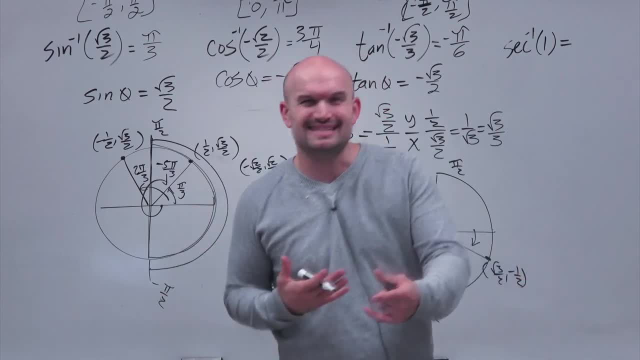 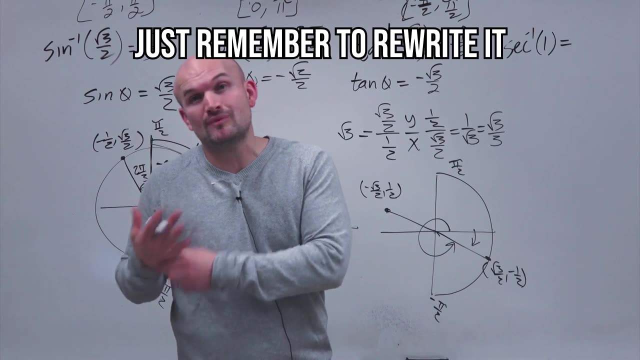 of secant, Like sometimes it gets confusing. It's like: well, again, secant is that the inverse, Like a lot of students will mix up secant with the inverse or the reciprocal. And again, my advice to you is just remember to rewrite it as a equation and then use it in terms 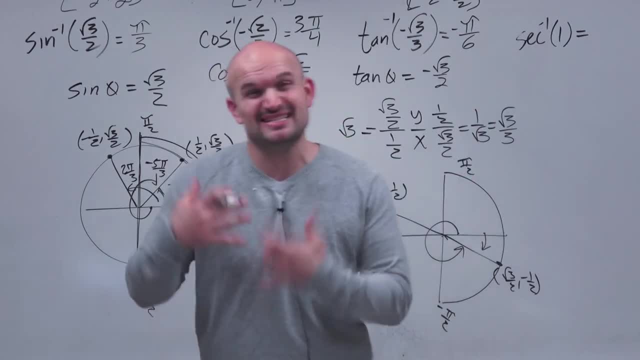 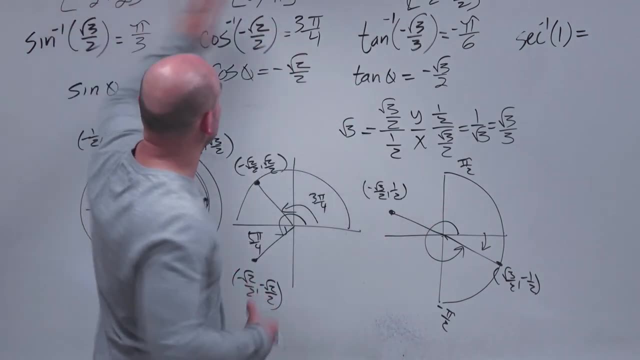 of cosine, Because we don't have in my notes. in my class we didn't talk about the restrictions of secant and looking at the graphs. We just looked at the graphs of these three functions to understand where, why these restrictions make sense. 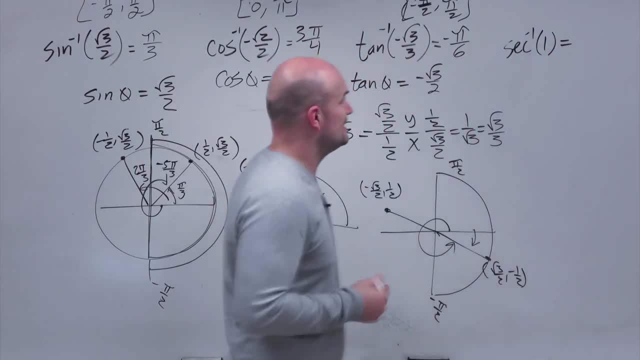 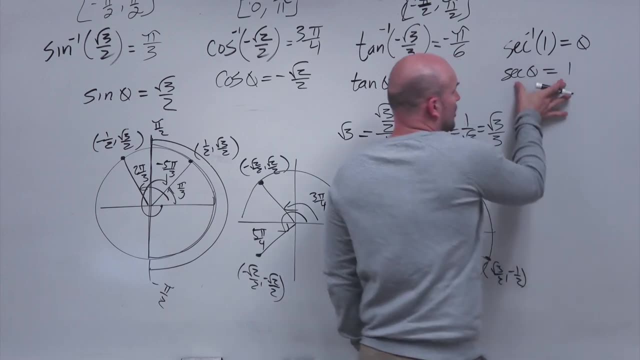 Well, for secant, again, if we think about this, we say secant of theta minus 1, is it even going to equal some angle? So therefore, the secant of some angle has to equal 1.. Well, again, I can take this equation and I can rewrite this as the cosine of theta. 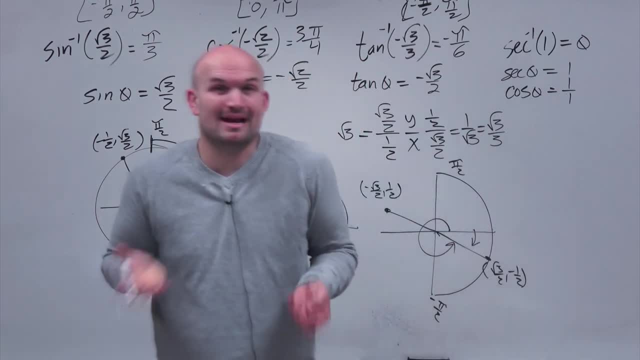 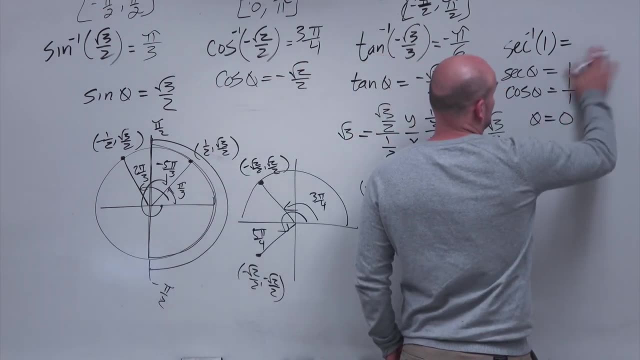 is equal to 1 over 1.. Well, this is kind of nice, because now it's saying: well, what angle produces cosine of what angle is 1? And that angle is just equal to 0.. So there you go, ladies and gentlemen.